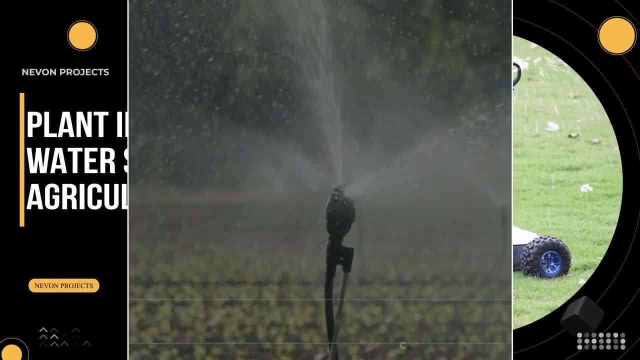 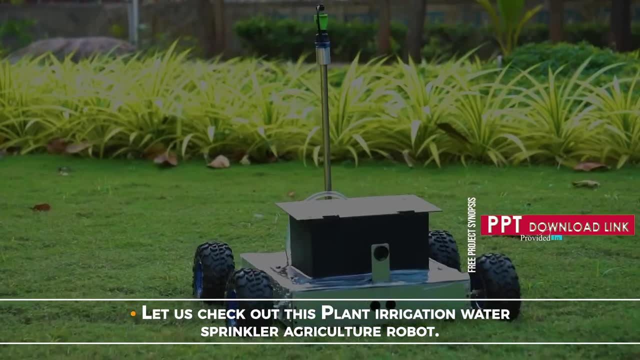 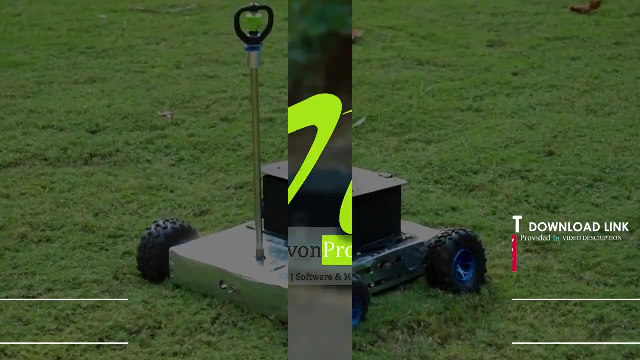 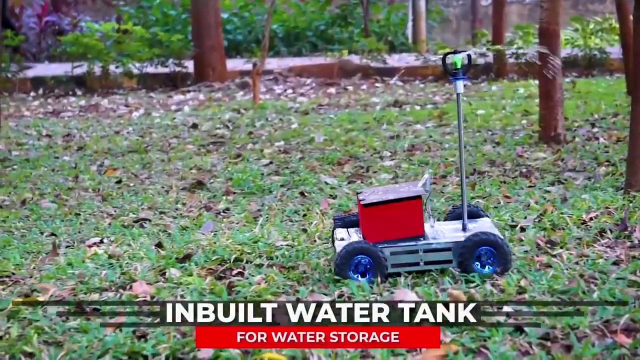 Plant Irrigation Water Sprinkler Agriculture Robot. Irrigation is the most important practice in the daily agriculture sector. Let us check out this Plant Irrigation Water Sprinkler Agriculture Robot. This robot is programmed to provide the correct amount of irrigation to the plants. 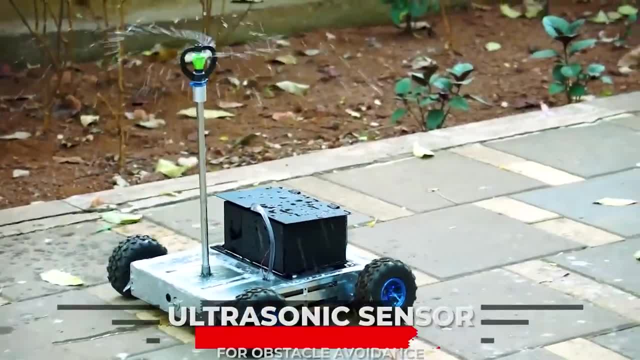 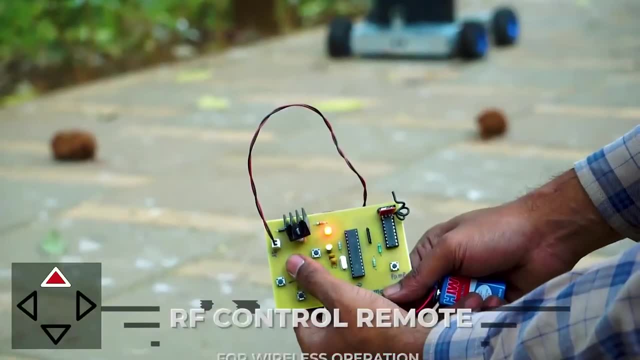 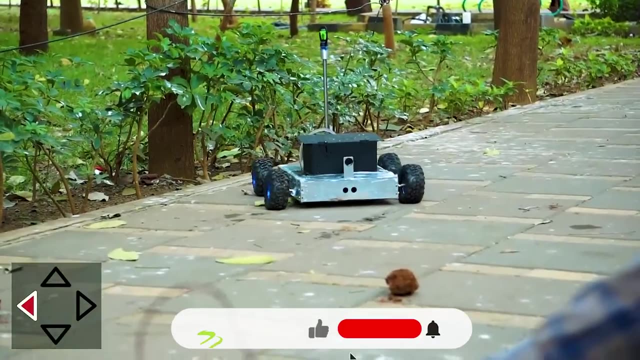 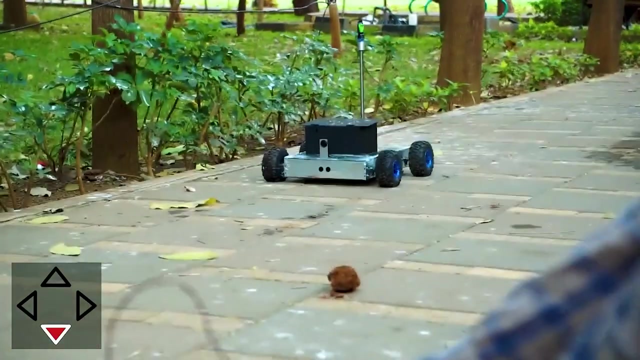 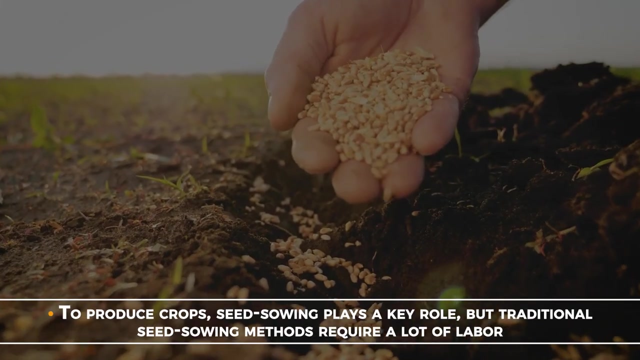 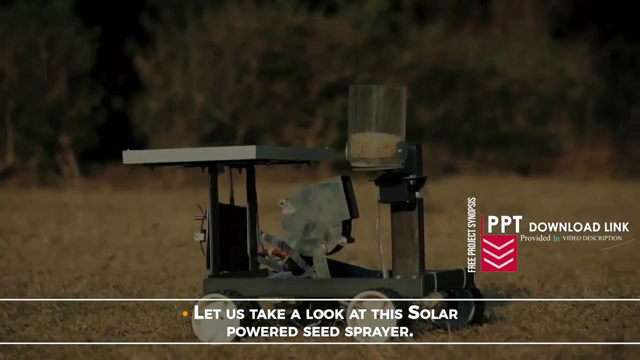 Plant Irrigation Water Sprinkler. Agriculture Robot. Design and Manufacturing of Solar Powered Seed Sprayer. Machine To produce crops, seed sowing plays a key role, But traditional seed sowing methods require a lot of labour. Let us take a look at this Solar Powered Seed Sprayer. 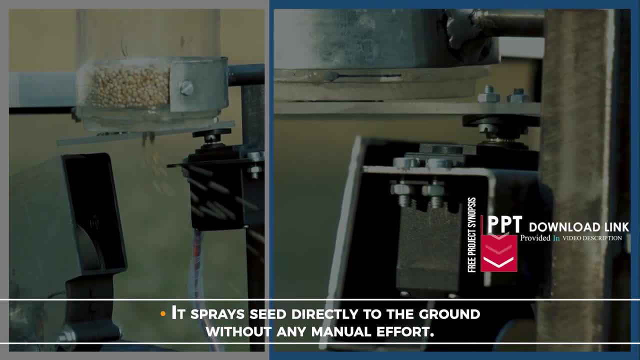 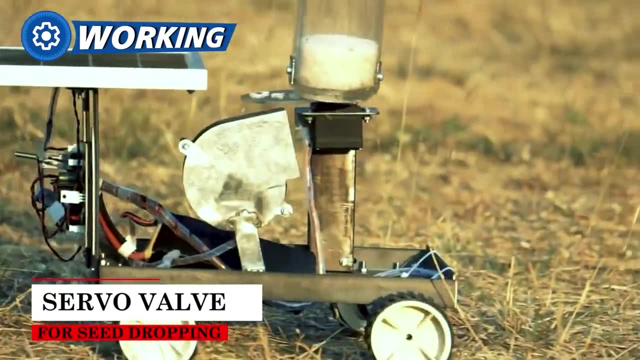 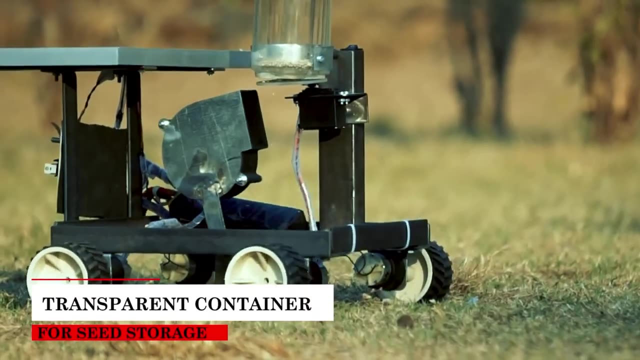 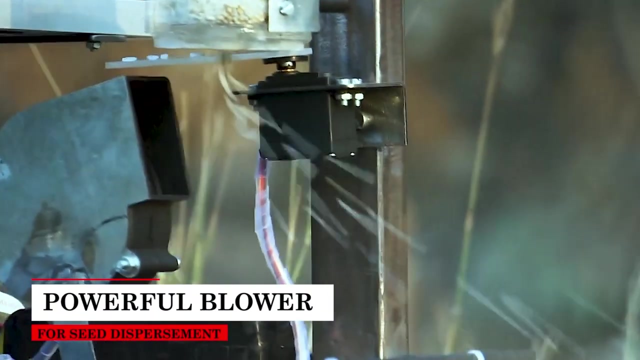 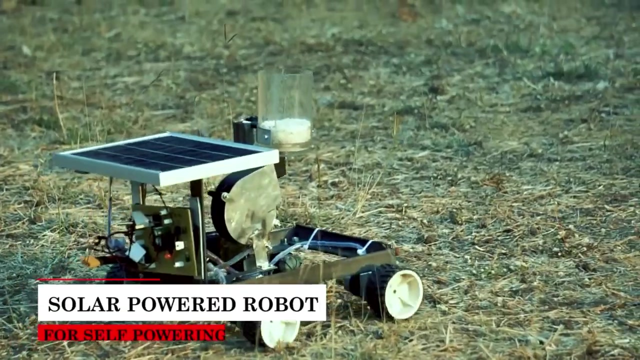 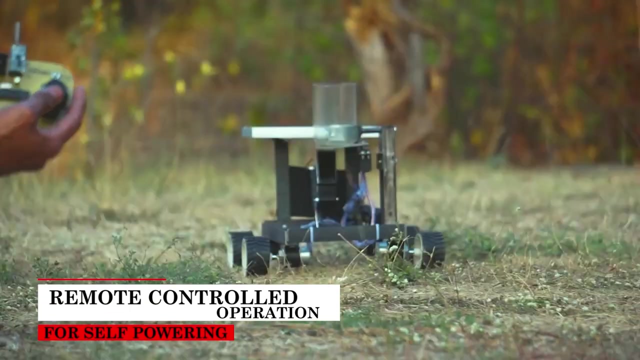 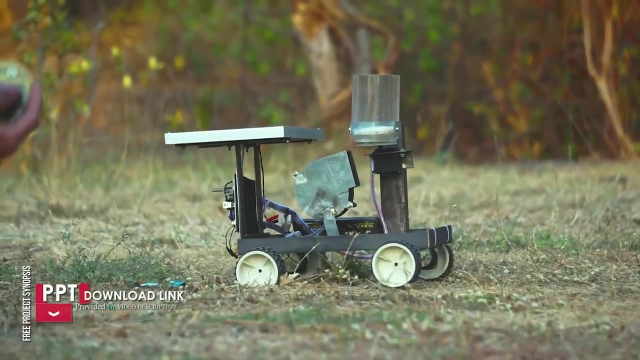 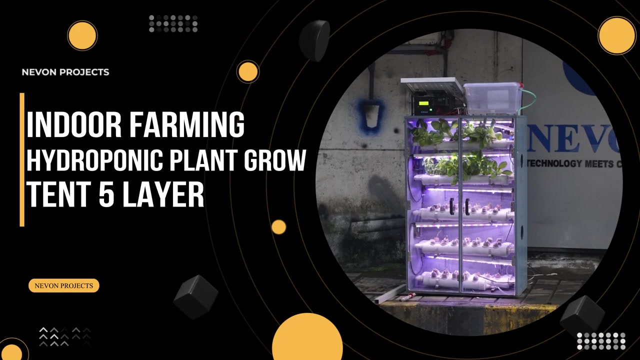 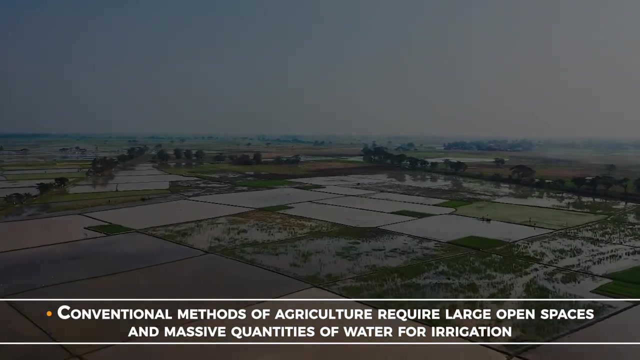 It sprays seed directly to the ground without any manual effort. ют Cord Wood Anaesthetics, fecil Communications- Music, Music, Music, Music, Music, Music, Music. Farming: Hydroponic Plant Grow Tent. Conventional methods of agriculture require large open spaces and massive quantities of water for irrigation. 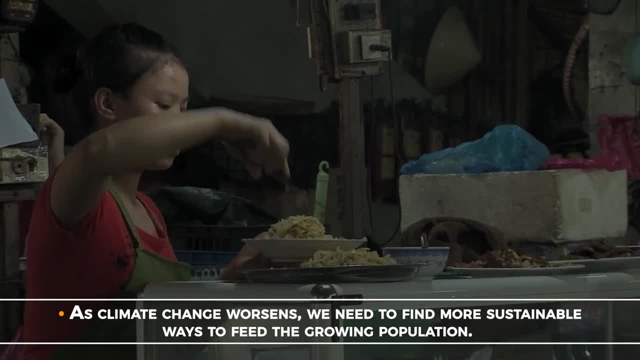 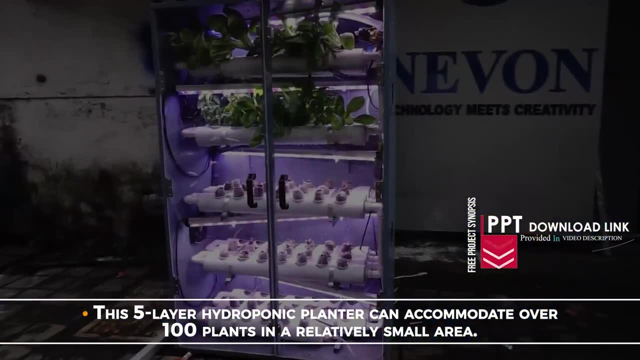 As climate change worsens, we need to find more sustainable ways to feed the growing population. This 5-layer hydroponic planter can accommodate over 100 plants in a relatively small area. Similarly, we have a single and a 3-layer hydroponic plant grow chamber. 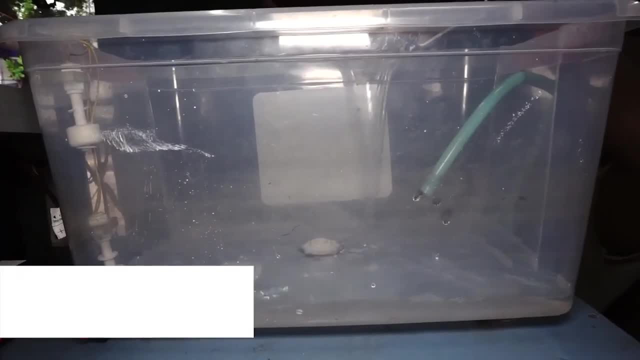 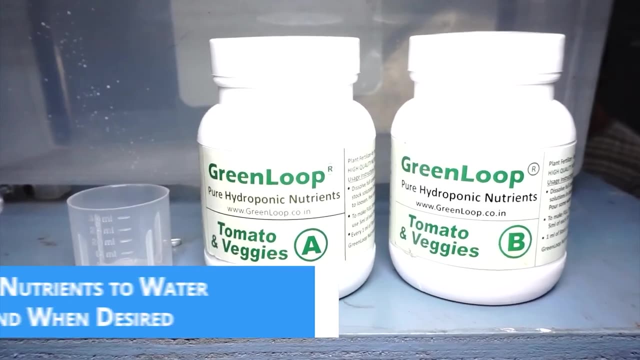 To be able to socio-economically and economically use the new hydroponic plant, we need to create a new center of growth which would be biologically and biologically developed. When the hydroponic plant is planted, it will have a completely different structure. 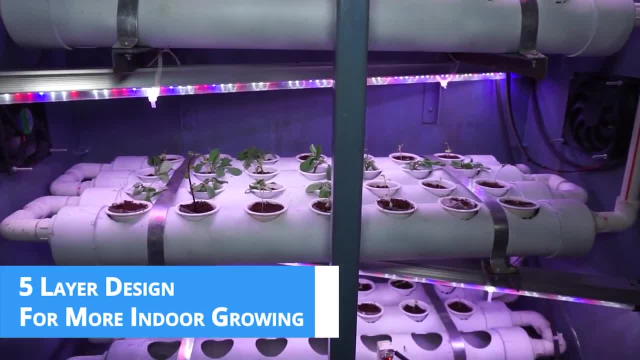 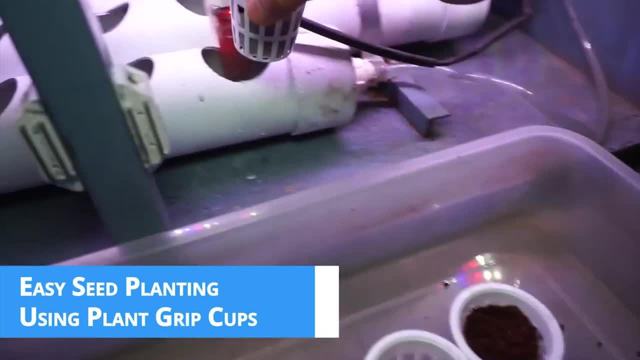 This is an example of the hydroponic plant grow chamber. The existing hydroponic plant is ours. as we can see from the plant structure, one single hydroponic plant we have. This is one of the three hydroponic falou plants. 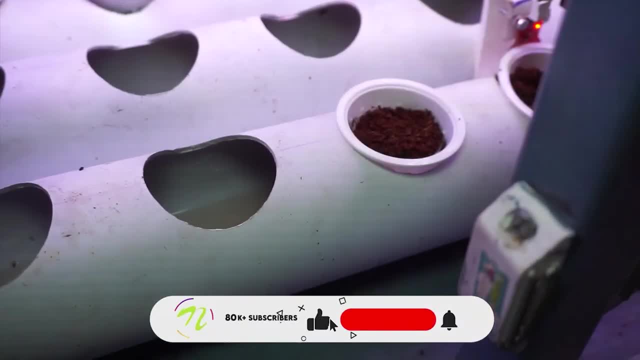 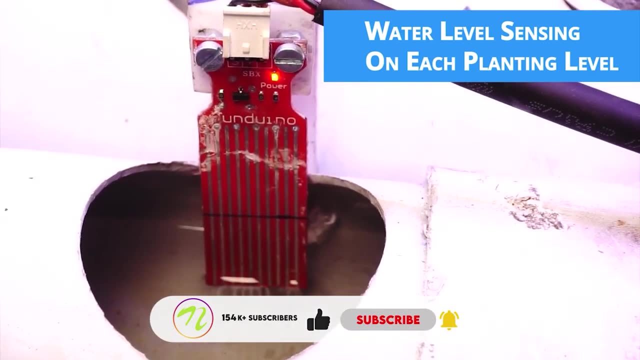 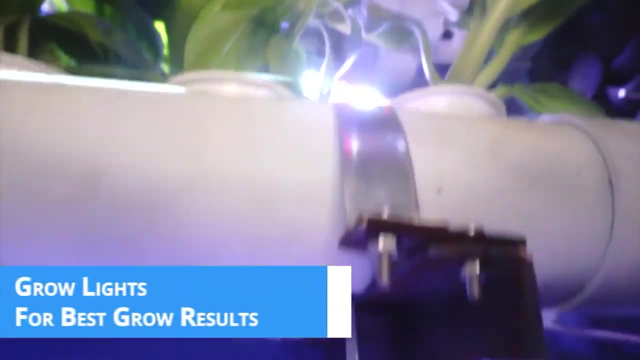 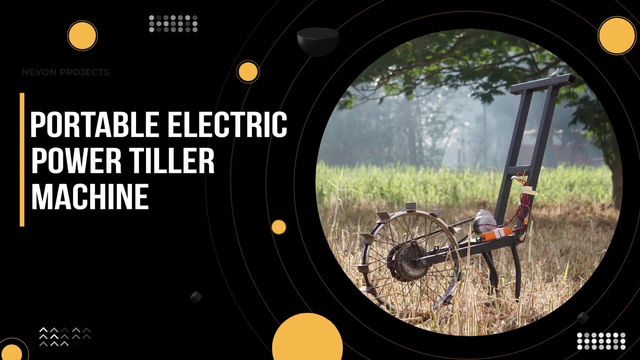 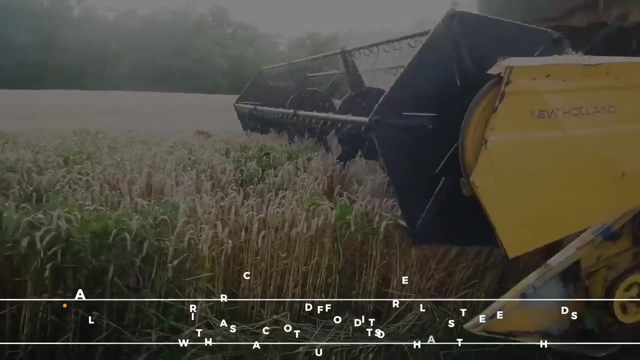 One of the three hydroponic plants is ours, As we can see from the plant structure: Poletable Electric Power Tiller Machine. Manual farm tilling is one of the most labor-intensive operations in agriculture. Also, many farmers cannot afford to replace these methods with a tractor due to its high cost. 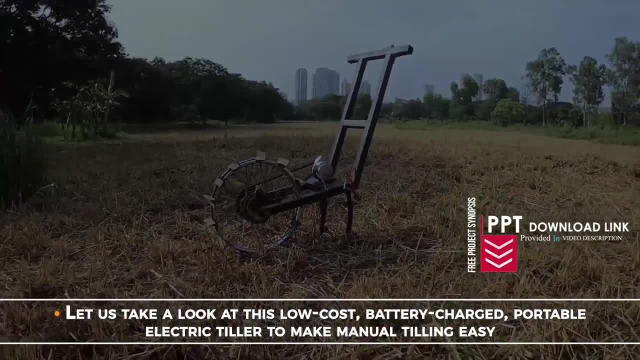 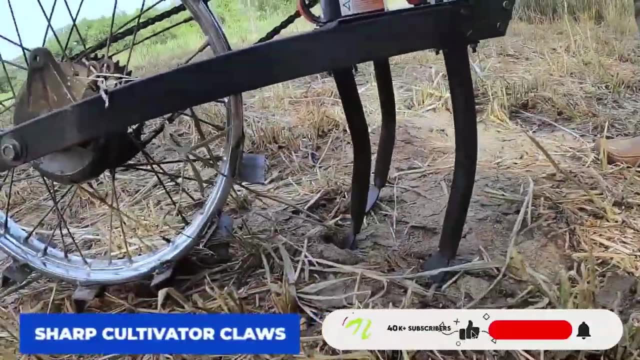 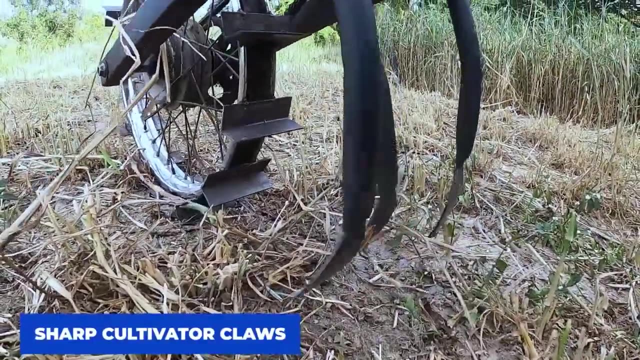 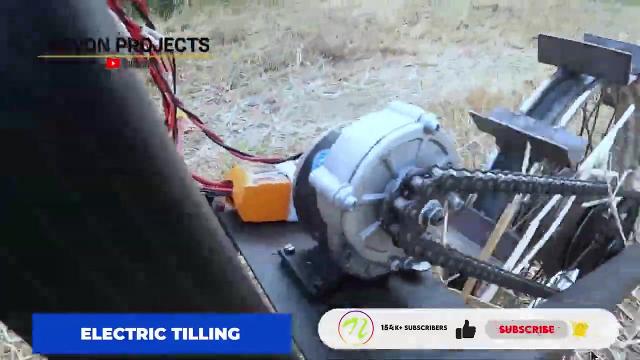 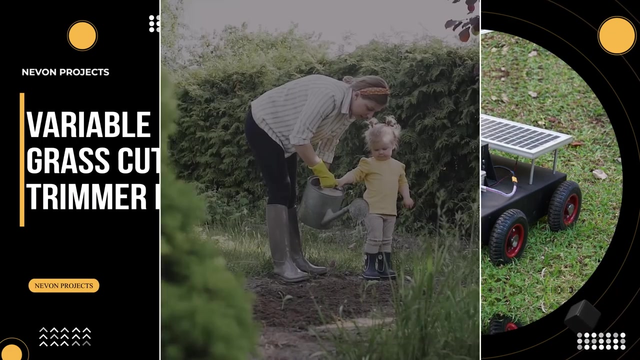 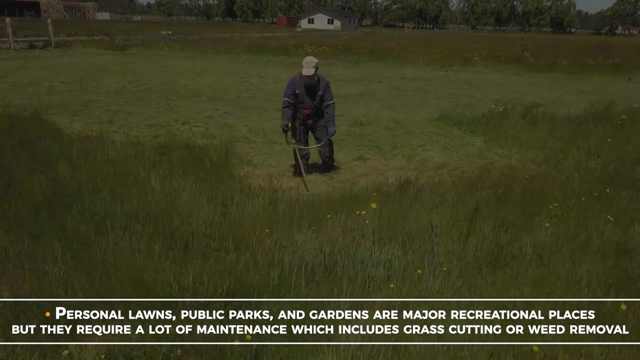 Let us take a look at this low-cost battery-charged potable electric tiller to make manual tilling easy. Variable Head Solar Grass Cutter, Weed Trimmer Robot. Personal lawns, public parks and gardens are major recreational places, but they require a lot of maintenance, which includes grass cutting or weed removal. 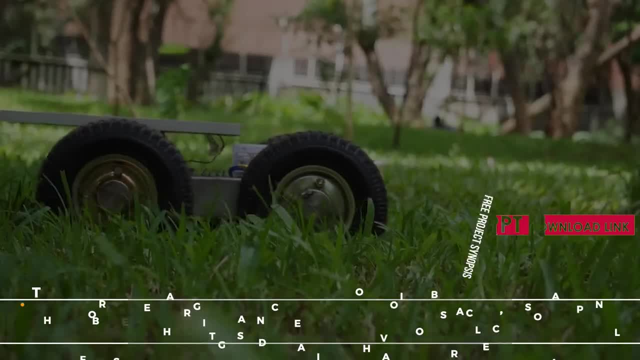 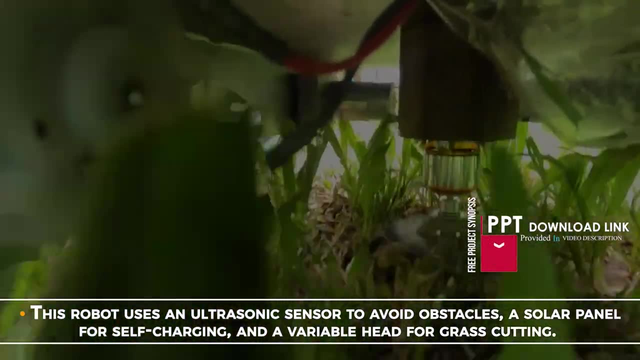 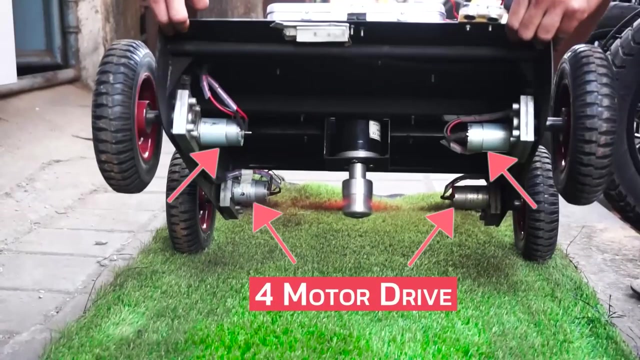 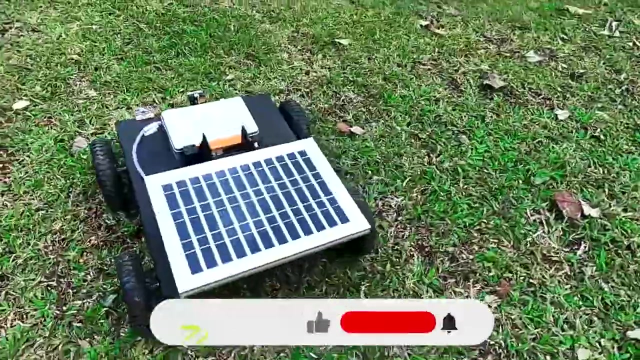 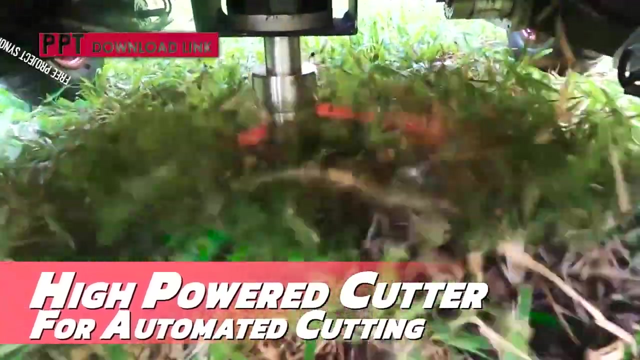 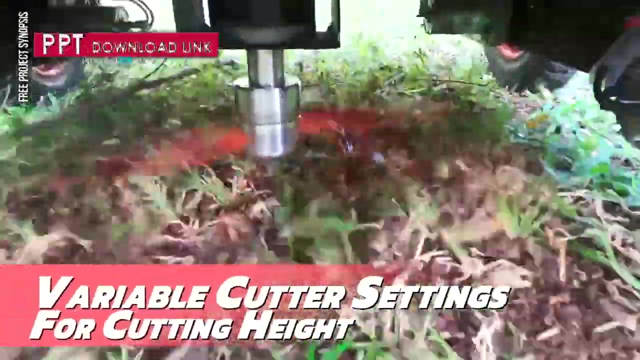 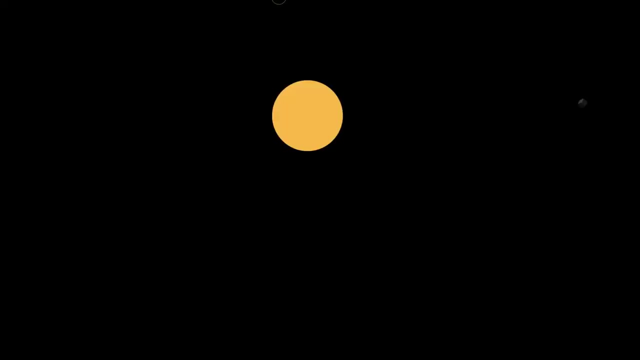 Let us check out this Variable Head Solar Grass Cutter Robot. This robot uses an ultrasonic sensor to record obstacles, a solar panel for self-charging and a variable head for grass cutting. Variable Head Solar Grass Cutter. Weed Trimmer Robot. Automatic Irrigation System. 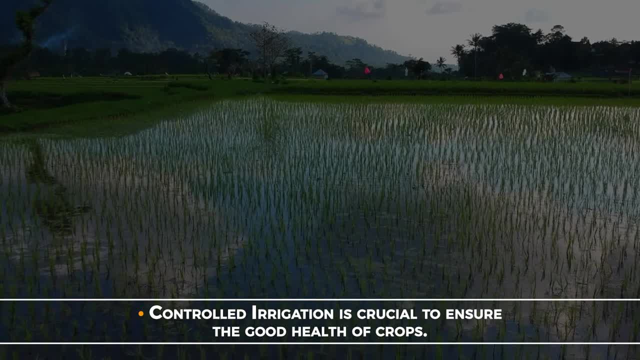 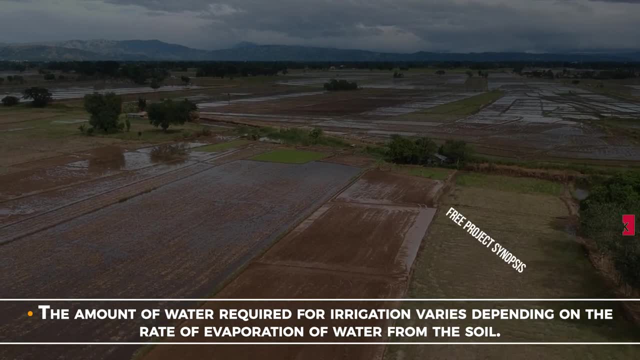 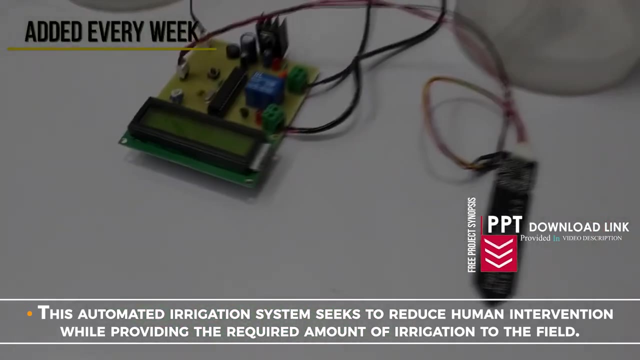 Controlled irrigation is crucial to ensure the good health of crops. The amount of water required for irrigation varies depending on the rate of evaporation of the water from the soil. This automated irrigation system seeks to reduce human intervention while providing the required amount of irrigation to the plant. 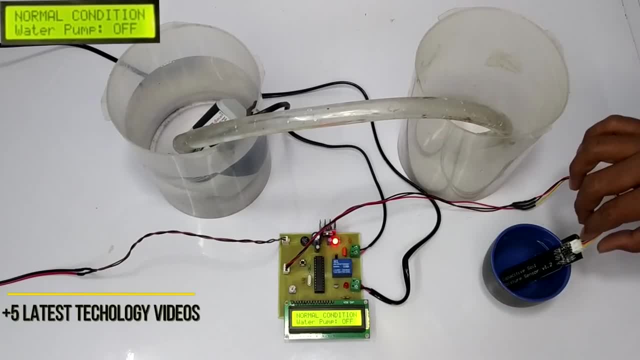 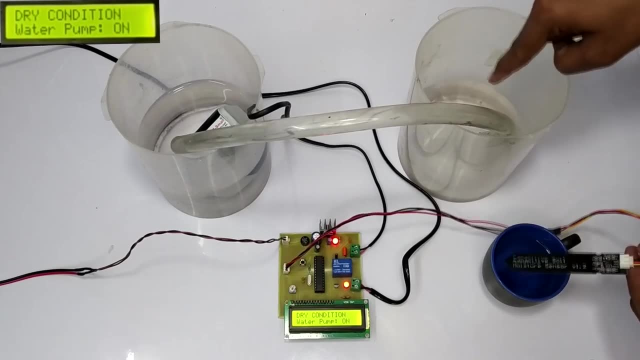 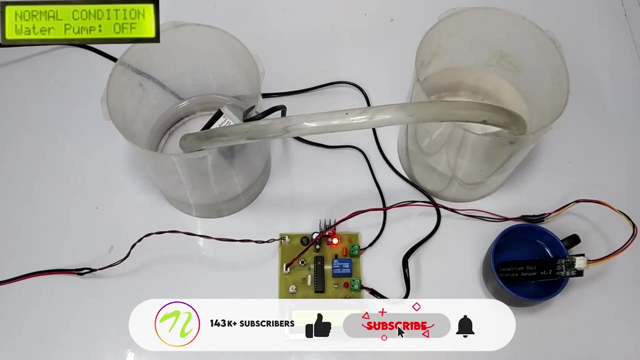 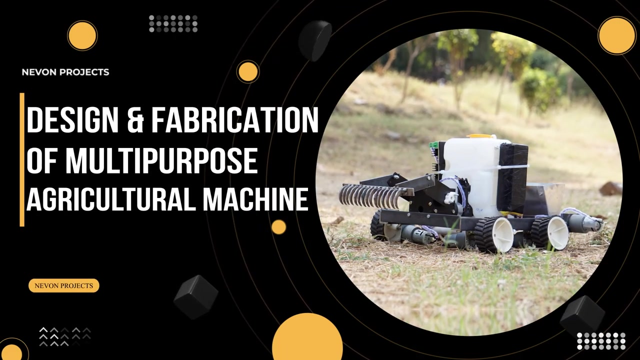 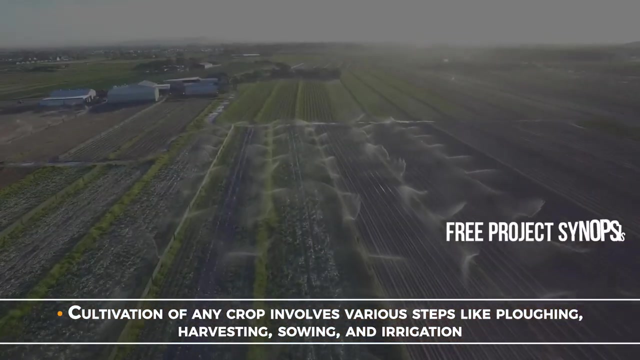 Variable Head- Solar Grass Cutter. Weed Trimmer Robot- Weed Trimmer Robot. Design and Fabrication of Multi-Purpose Agriculture Machine. Cultivation of any crop involves various steps like plowing, harvesting and recycling, harvesting, sowing and irrigation. Let us check out this multi-purpose agriculture robot which can perform a variety of agricultural. 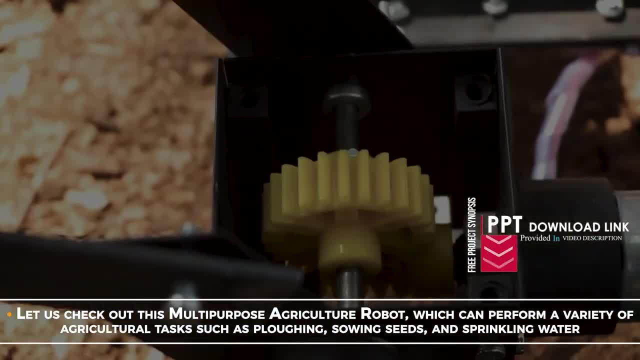 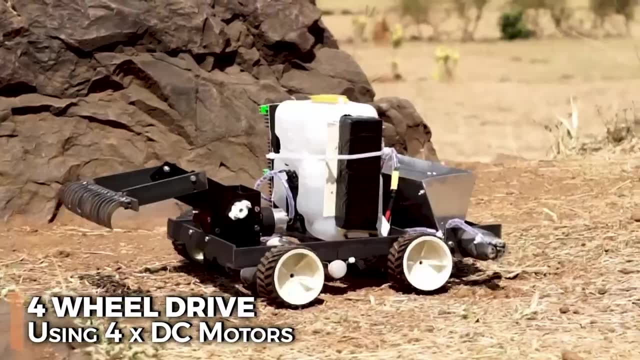 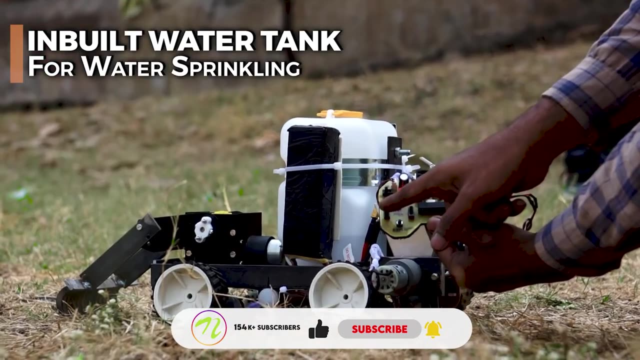 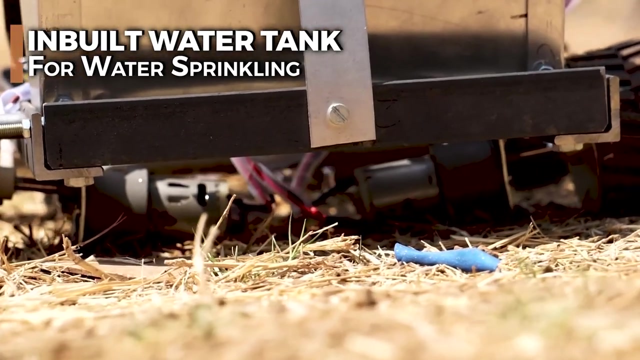 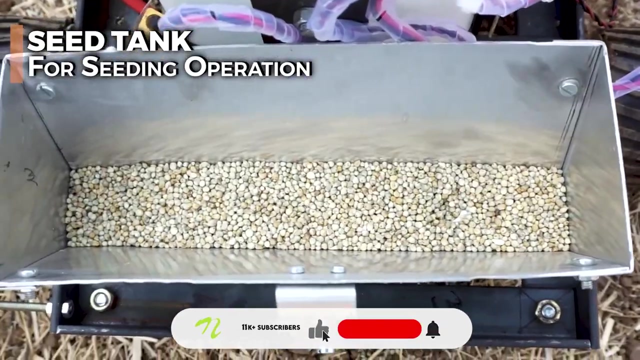 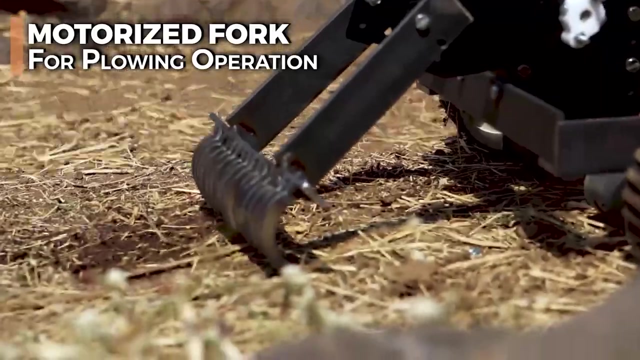 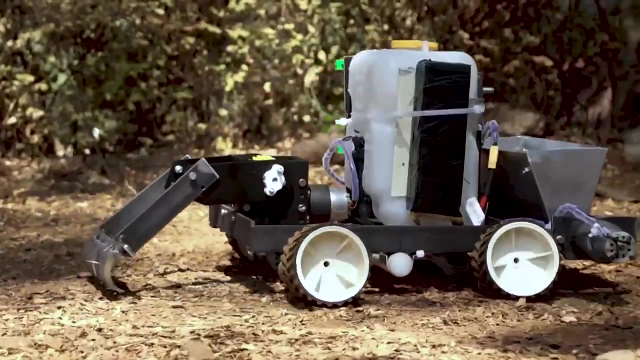 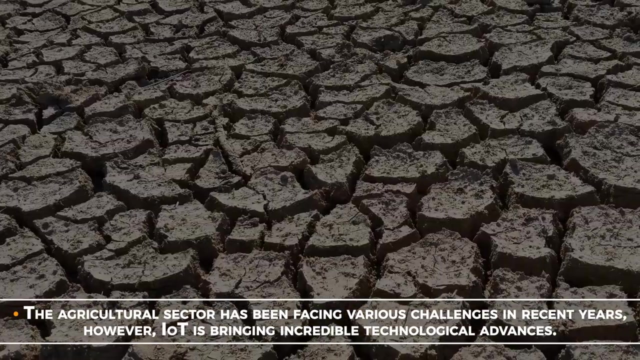 tasks such as ploughing, sowing seeds and sprinkling water. IOT-based Smart Agriculture Monitoring System. the agricultural sector of India is one of India's leading agricultural sector has been facing various challenges in recent years. However, IOT is bringing incredible technological advances. 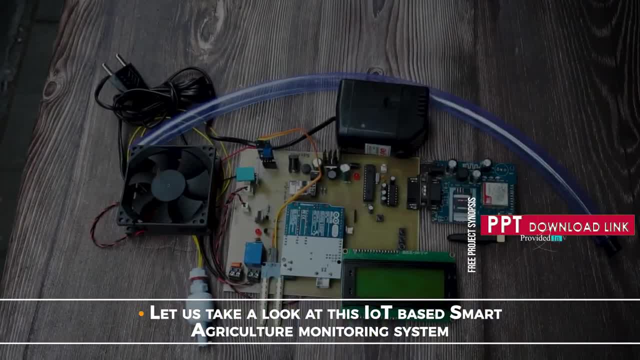 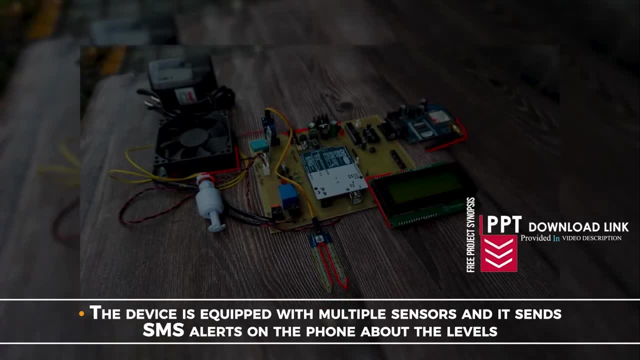 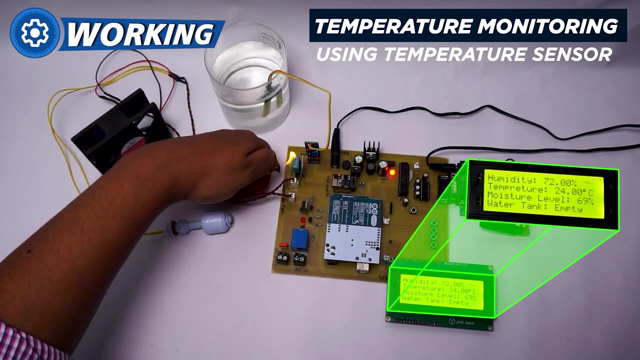 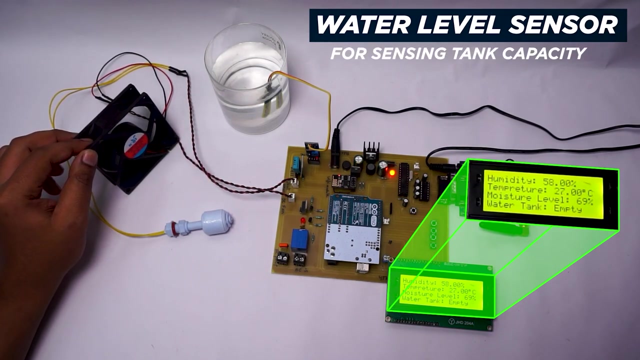 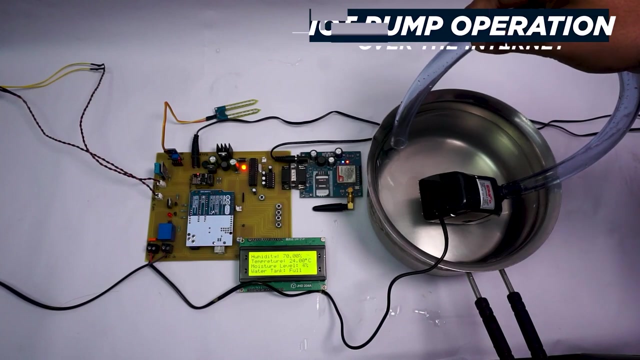 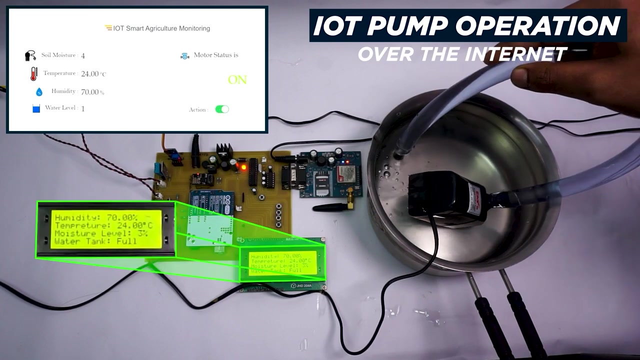 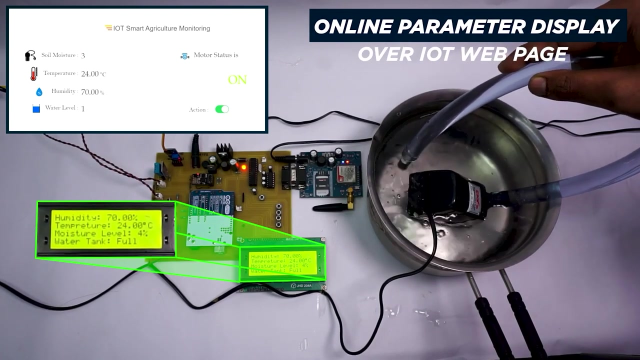 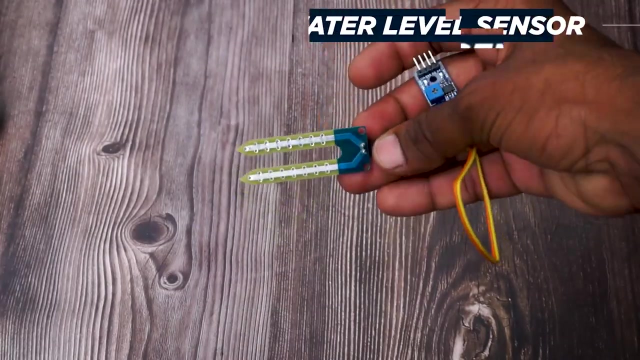 Let us take a look at this IOT-based Smart Agriculture Monitoring System. The device is equipped with multiple sensors and it sends SMS alerts on the phone about the levels. The device is equipped with multiple sensors and it sends SMS alerts on the phone about the levels.